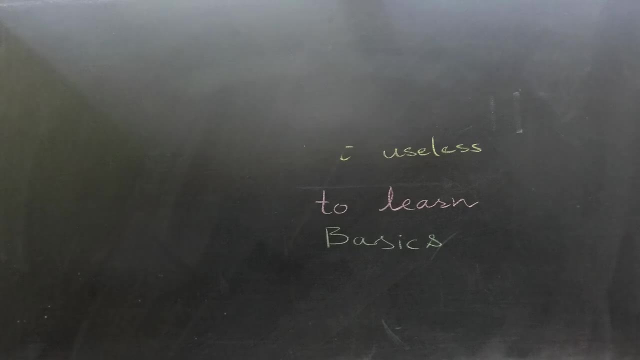 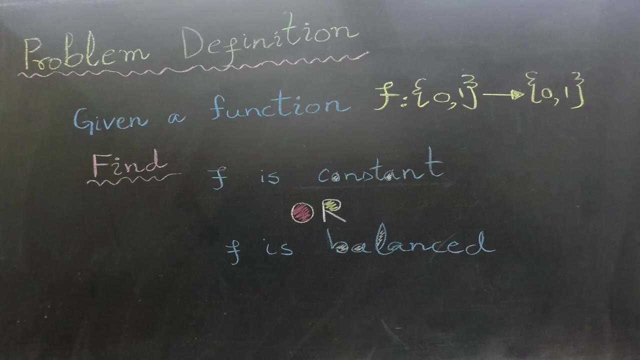 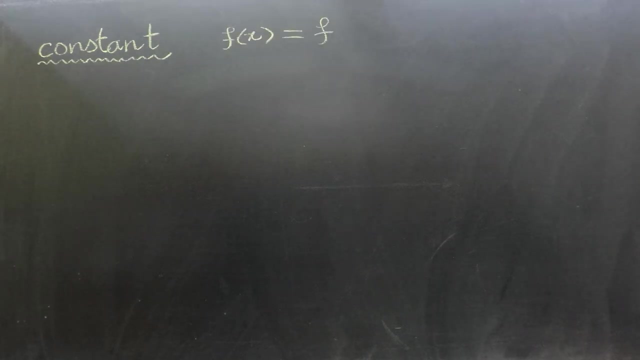 your feet wet. Let's start with the problem definition. Given a function f that takes a single bit s input and yields a single bit output, our goal is to determine whether the function f is equal to or equal to zero. A function is called constant if it produces the same output regardless of the input it. 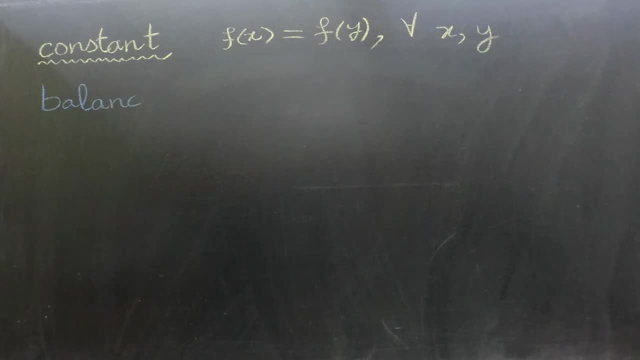 receives. In contrast, a function is considered balanced if its yield are zero for half of the possible inputs and one for the other half. Let's consider all the cases for both constant and balanced. When the function is constant for inputs zero and one, it will either always produce all. 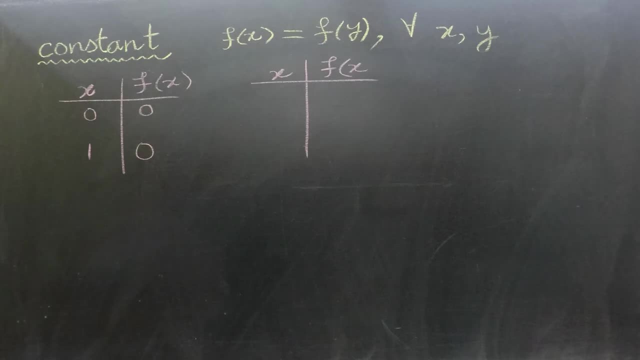 zeroes as output, referred to as case 1, or all ones as output- case 2.. When the function is balanced, we have two decisions. The first is to determine the value of the function f and the second is to determine the value of the function f. The second is to determine the value of the function f. The third is to determine the value of the function f. The fourth is to determine the value of the function f. The fifth is to determine the value of the function f. The next consideration is that for a function f we do not need two additional cases. 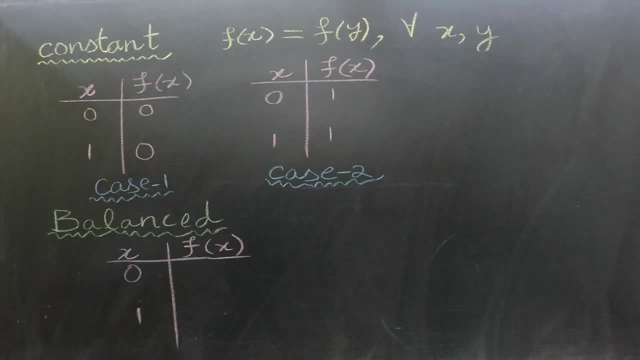 In one scenario, for inputs 0 and 1, it will yield the same output of 0 and 1.. Case 3: Alternatively, for inputs 0 and 1, it will yield 1 and 0, which we will call case 4.. 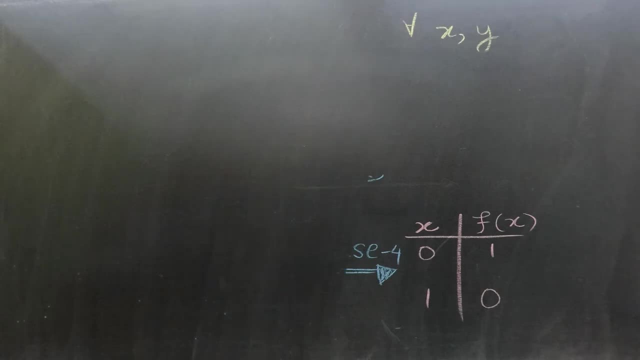 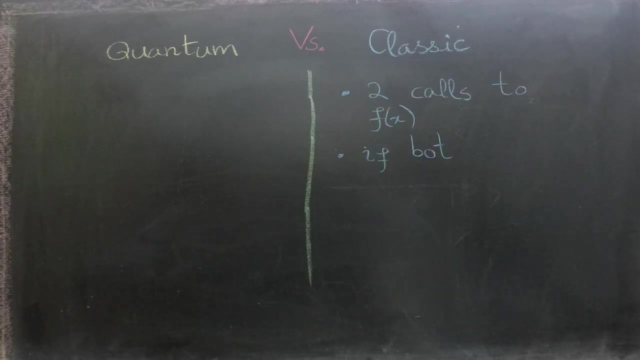 The following case will be case 4.. We will use these cases later, cases later in the algorithm To solve this problem. on a classical computer the function f must be called twice. It is considered constant when both outputs are the same, otherwise it is termed as balanced. 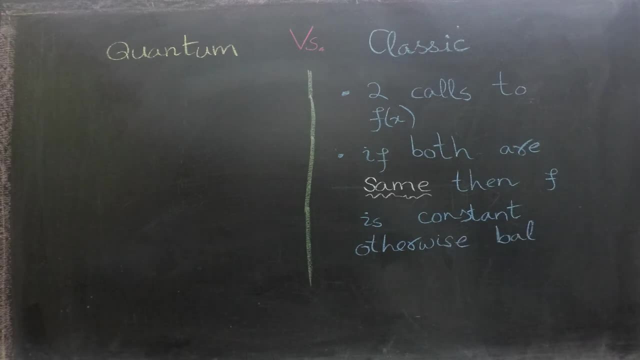 The key emphasis here is making two function calls for classical computation. In contrast, in Deutsch Algorithm the function is called only once, as it employs the superposition of all possible inputs. This superposition results in speeding up the quantum algorithm. Now let's draw the quantum circuit for Deutsch Algorithm. 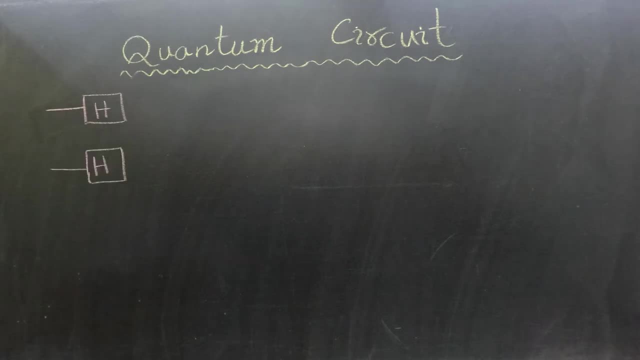 It takes inputs cat0 and cat1, and these inputs are processed by Hadamard gates. The results are then passed on to the UF gate, which has been explained in detail in the previous video. Now let's draw the quantum circuit for Deutsch: Algorithm. 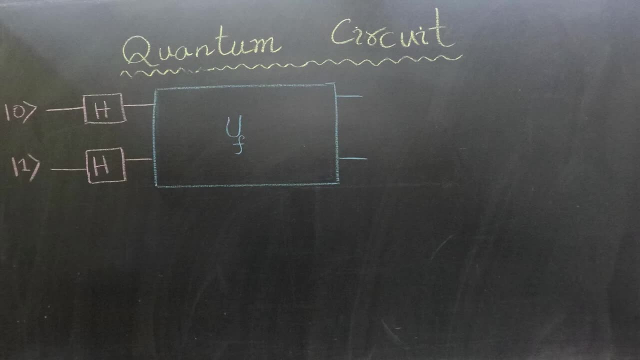 The results are then passed on to the UF gate, which has been explained in detail in the previous video. Please watch it first, in case you have missed it. The UF gate takes input catx and caty, resulting in output of catx and cat. fx xor y. 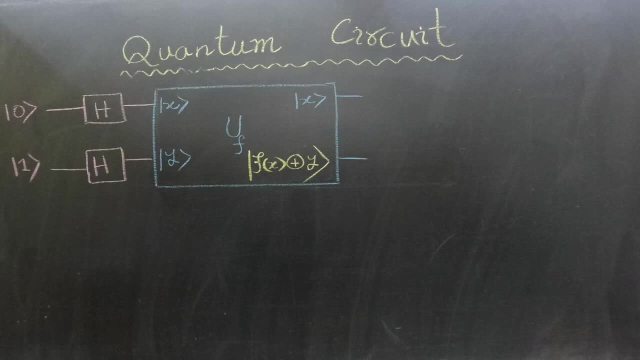 Following the application of UF gate, a Hadamard gate is once again applied, but solely to the first qubit. Subsequently, the first qubit is measured. Now here is the claim: If we measure zero on the first qubit, the function must be constant. 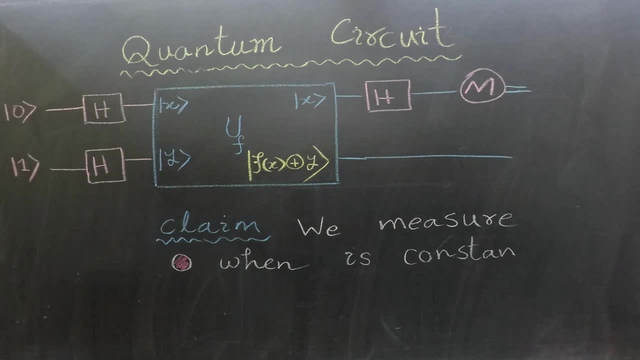 Otherwise it is balanced. Let's validate this claim. To aid in our verification, we have divided the circuit into four different stages. The first stage is labeled as catx1,, the second stage as catx2, the third stage as catx3,. 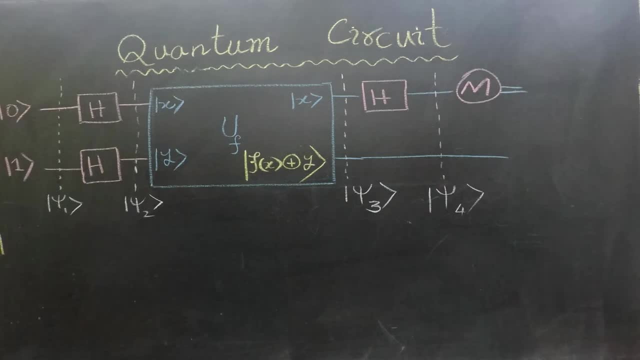 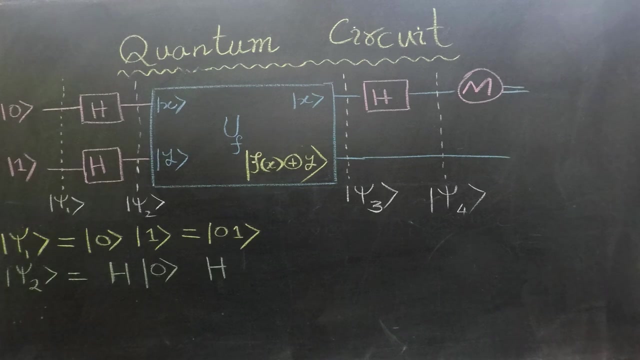 and the final stage as catx4.. Catx1 is equal to the tensor product of cat0 and cat1, which can also be represented as cat01.. To calculate catx2, we apply Hadamard gate to the both qubits. 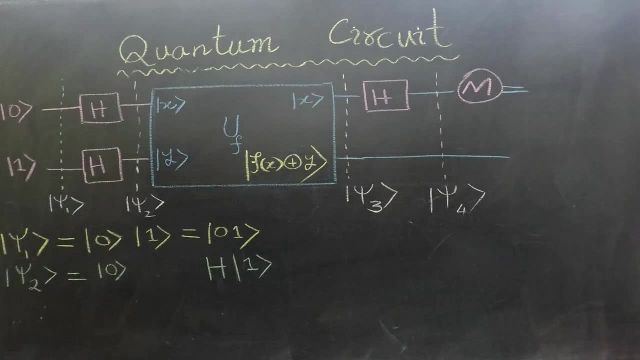 Applying a Hadamard gate to cat0 results in cat0 plus cat1 divided by the square root of 2.. Similarly, applying a Hadamard gate to cat1 results in cat0 minus cat1 divided by the square root of 2.. 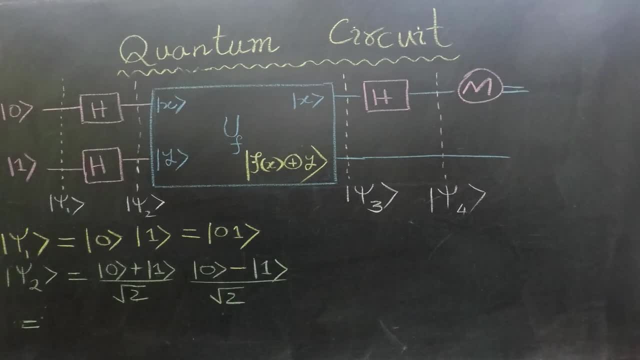 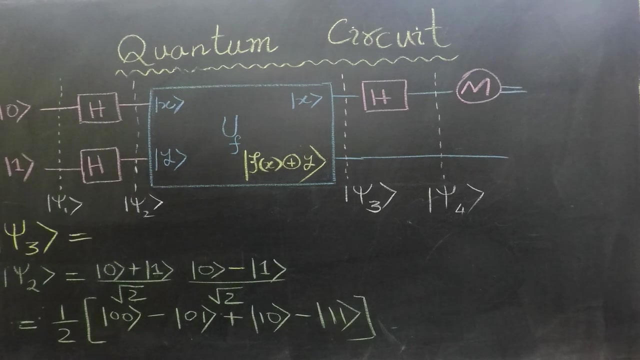 Cat. side 2 can be simplified to 1 over 2 times cat00 minus cat01, plus cat01 divided by the square root of 2.. Let's start the calculation. Let's start the calculation. plus cat10 minus cat11.. To calculate catSide3, we apply ufgate to catSide2.. 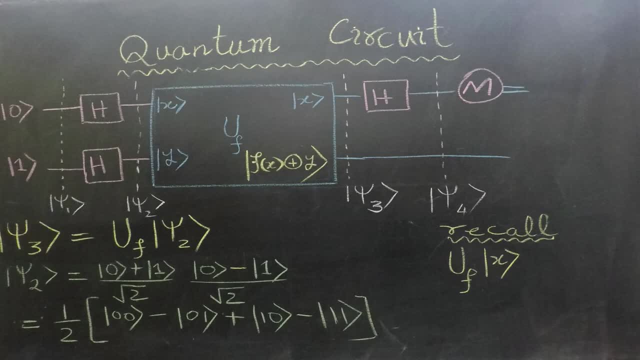 Remember, ufgate takes catX and catY as inputs and yield an output of catX and catFFX, XORed with Y. First, both X and Y are equals to 0.. Applying ufgate will give us cat0 and catFFXXORed with 0.. 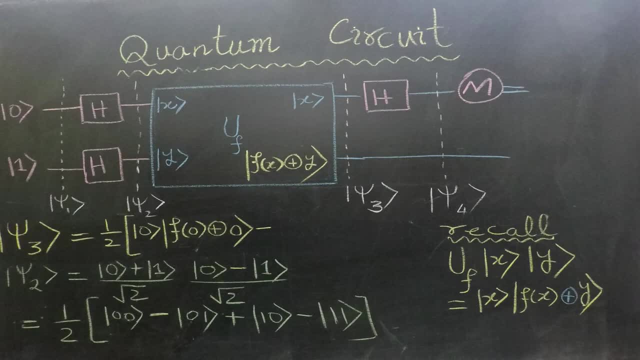 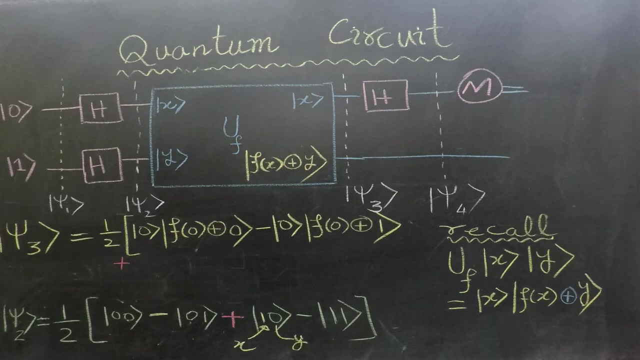 The minus sign remains unchanged. Now, when X is cat0 and Y is cat1, applying ufgate produces cat0 and catFFXXORed with 1.. Next, with X as cat1 and Y as cat0, applying ufgate results in cat1 and catFFXXXORed with. 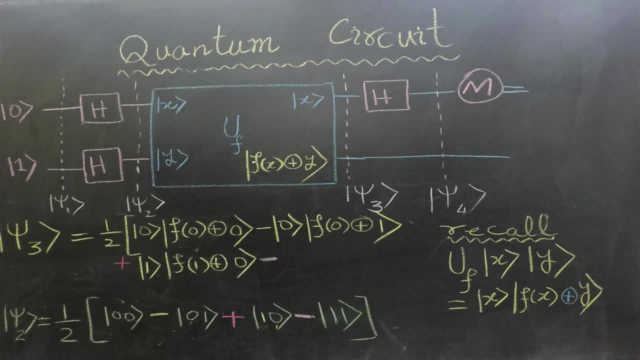 0.. Finally, when X is cat1 and Y is also cat1, applying ufgate transformed it into cat1.. Finally, when X is cat1 and Y is also cat1, applying ufgate transformed it into cat1.. 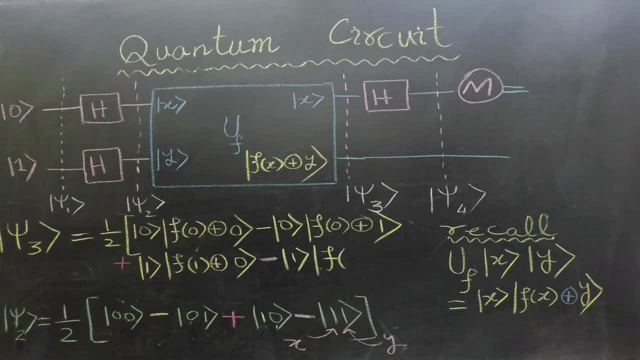 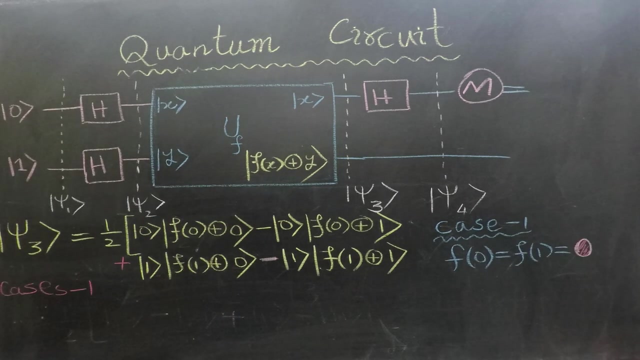 cat 1 and cat f of 1 XOR with 1.. Recall that in case 1, both f0 and f of 1 are equals to 0.. Substituting these values for f of 0 and f of 1 simplifies cat psi 3 as. 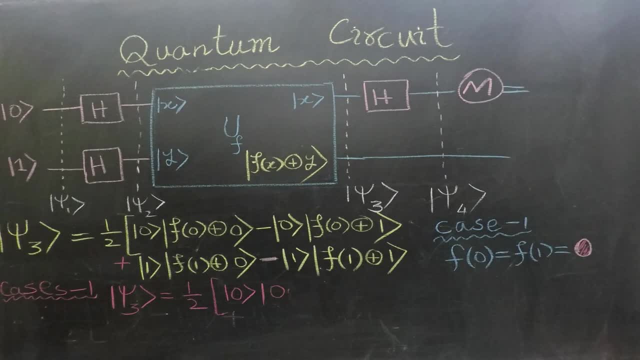 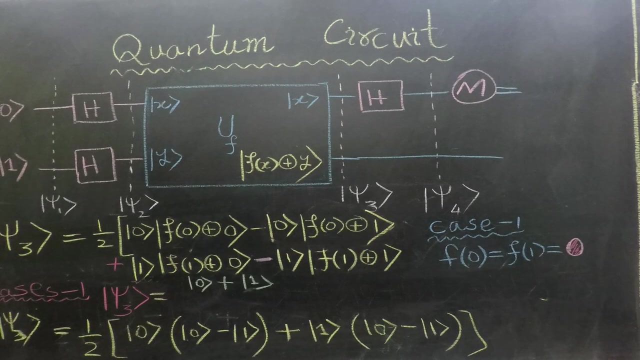 shown here. Next, we factor out cat 0 from the first two terms and cat 1 from the last two terms. This transforms cat psi 3 into cat 0 plus cat 1, divided by a square root of 2.. Cat 0 minus cat 1. 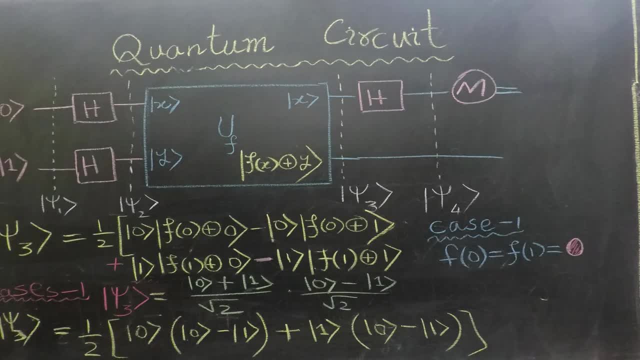 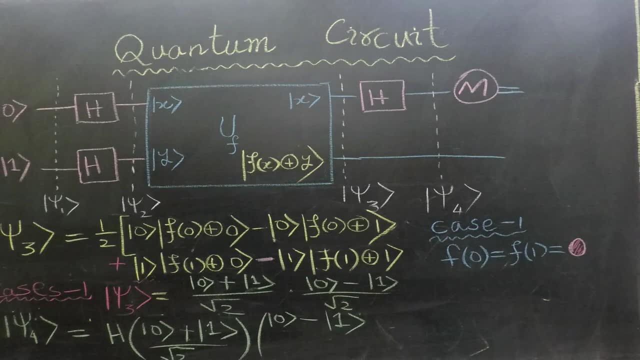 To calculate cat psi 4, we need to apply a Hadamard gate to the first qubit. It is important to note that the first qubit is in the state cat plus, which means that applying a Hadamard gate to it will result in cat 0.. Now when we measure the first qubit, we will get cat. 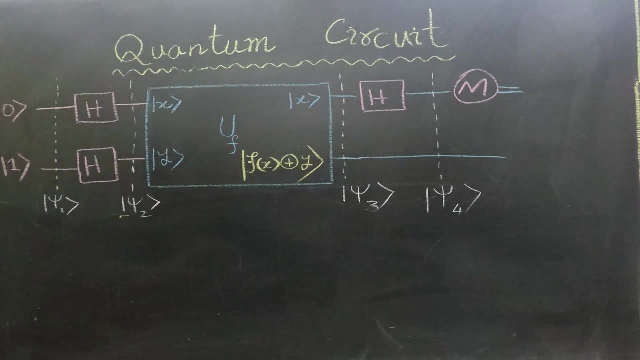 0 with 100% probability. Now let's look at the first qubit. Now, when we measure the first qubit, we will get cat 0 with 100% probability. In conclusion, when the function is constant in cat psi 3, the first qubit will be either: 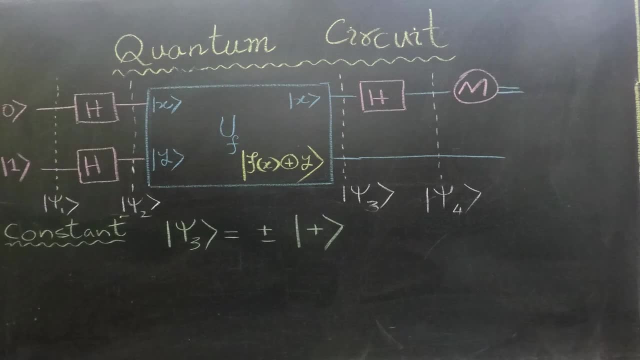 cat plus or minus cat plus and the second qubit will always be cat minus. For those who are unfamiliar, cat plus is represented as cat 0 plus cat 1, divided by the square root of 2, and cat minus is referred as cat 0 plus cat 1.. 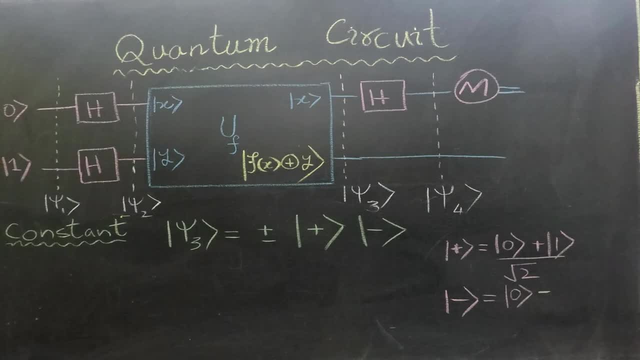 Now, if we'll calculate that, we will get, cat plus is represented as cat 0 plus cut 1 divided by the TRAGE. Applying a Hadamard gate to the first qubit of cat plus will result in cat 0, which will be measured as 0 with 100% probability. Note that we do not have to worry about the 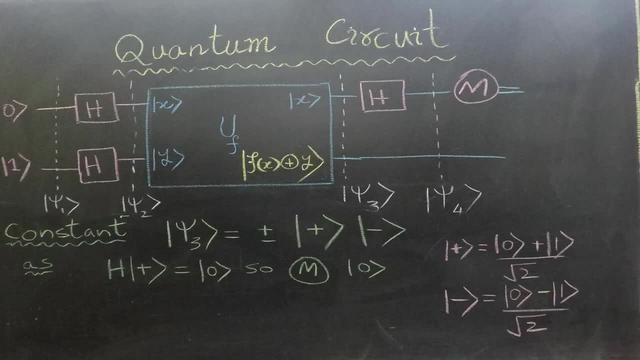 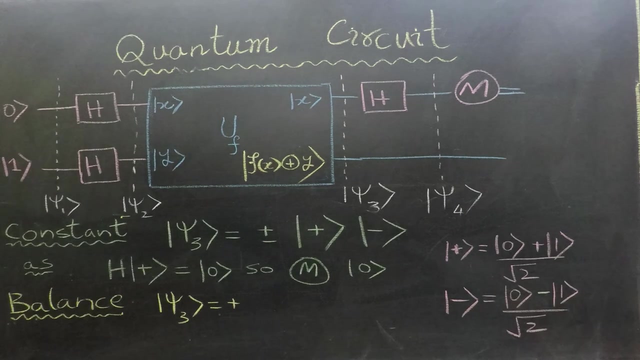 potential minus sign of cat 0. since its probabilities are the square of the amplitude, then it will still be measured as 0 with 100% probability. When the function is balanced in ket psi 3, the first qubit will be plus minus, ket minus and the second qubit will be ket minus. In ket psi 4, applying Hadamard: